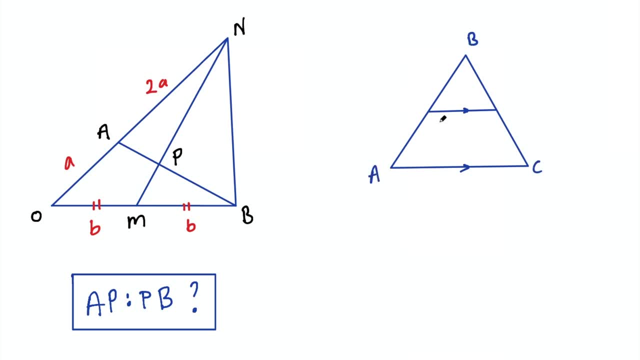 So, for example, if I have this triangle ABC and this line here divides AB in half. so let's say let's call this point X. so let's say AX equals XB, then it will also divide the other side in half. So these two lengths- let's say let's call this BY- will equal YC. So this is a. 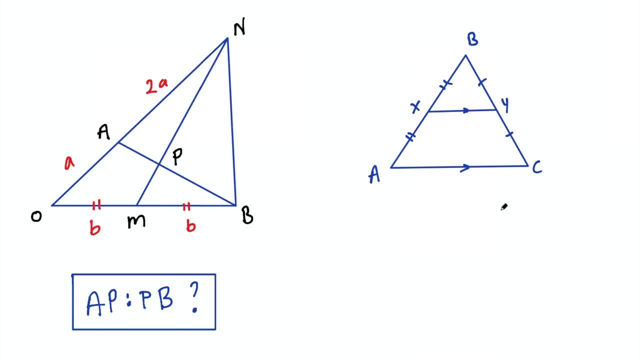 fact that you can prove using vectors if you like, or there's different ways to prove it, but yeah, so basically, if you have this line XY and it's parallel, in this example, to AC, whatever ratio it divides one side again, We'll divide the other side in the same ratio. Okay, so we're going to use that fact in this. 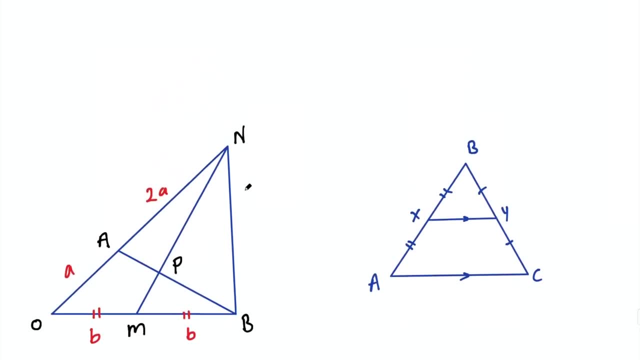 problem to solve it really quickly. So, firstly, we're going to draw a line parallel to MN, So we're going to draw a line from B that is parallel to MN, and this line just goes on forever, Okay. and then we're going to extend the line ON until it intersects with this line, Okay. 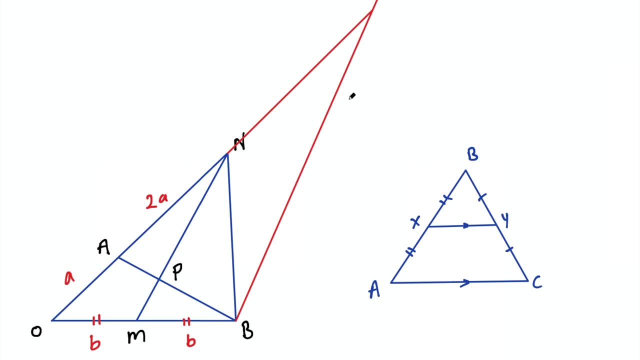 so so far, we are perfectly fine doing that. There's nothing wrong with saying this is parallel to MN and that we we will have a line from O that will intersect with this new line. Okay, so now notice this triangle O. let's call this point up here. X. Let's notice this triangle OXB, This line MN. 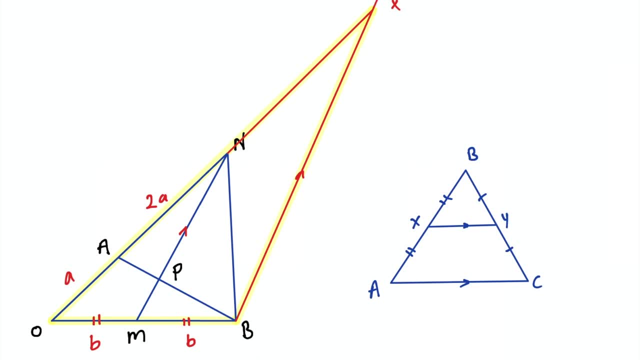 divides OB in half. so, using what we just talked about, it will also divide OX in half. So if we're calling OAA and AN2A, then this entire length is 3A. then NX will also be 3A because, as we said this: 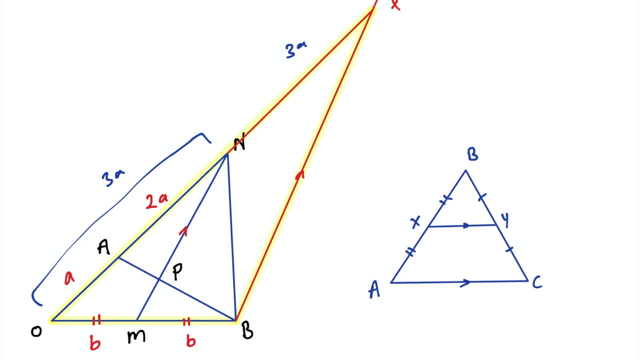 line MN must cut both sides of that triangle in half. And now notice a different triangle. Notice this triangle in here: AXB. So if we look at the line PN, well, if it's dividing the line AX in the ratio 2 to 3, then it must also